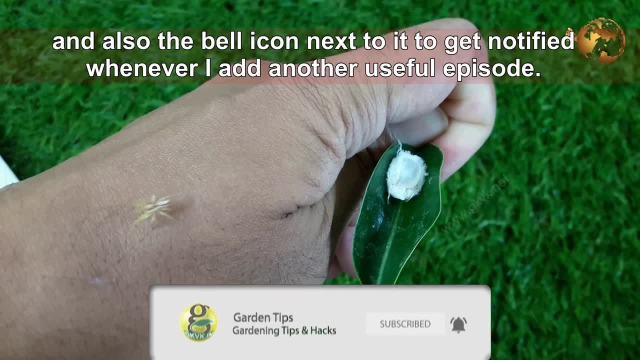 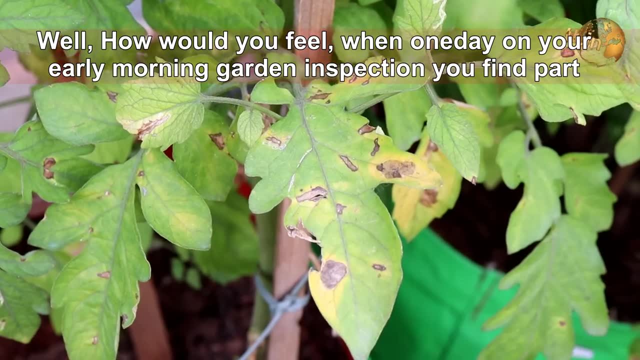 and also the bell icon next to it to get notified whenever I add another useful episode. Well, how do you feel when one day, on your early morning garden inspection, you find part of your garden disappeared while you slept or realize your flower buds are torn apart? 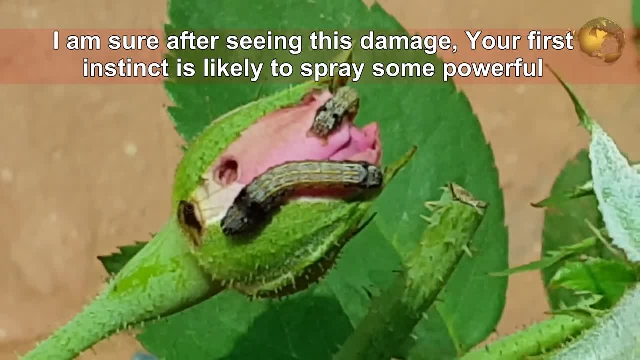 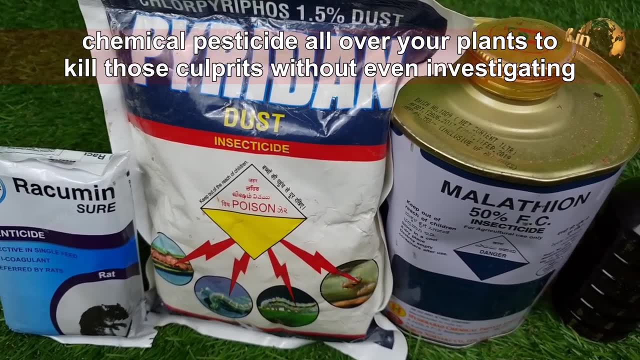 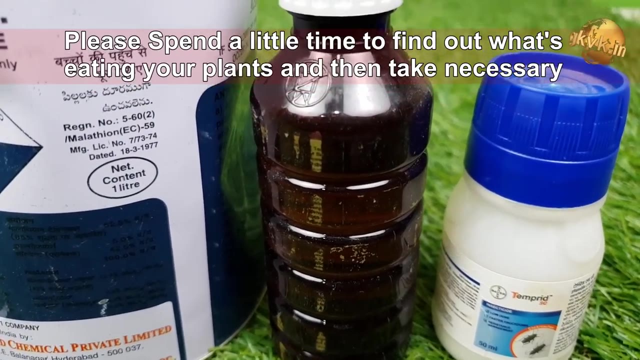 and are very badly damaged. I am sure after seeing this damage, your first instinct is likely to spray some powerful chemical pesticides all of your plants to kill those culprits, without even investigating further. This is not a right decision. Please spend a little time to find out what is eating your plants and then take necessary 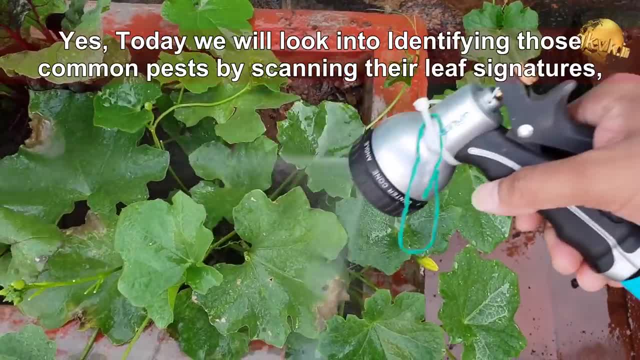 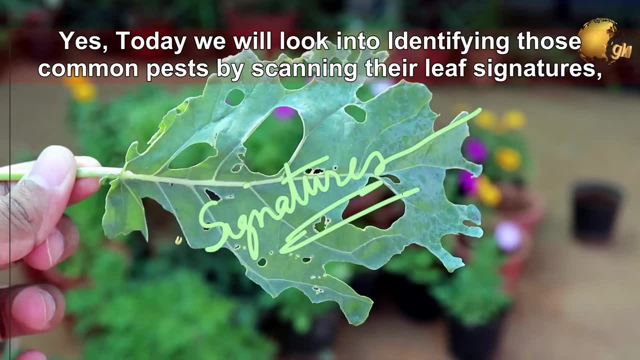 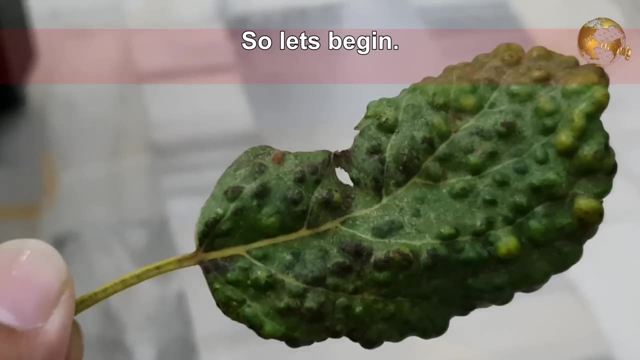 action particularly prescribed for that pest or insect. Yes, today we look into identifying those common pests by scanning their leaf signatures, ie the leaf damage pattern they leave after feeding on your plants. So lets begin. The first pattern is Chewed Leaves or Slime Trails. 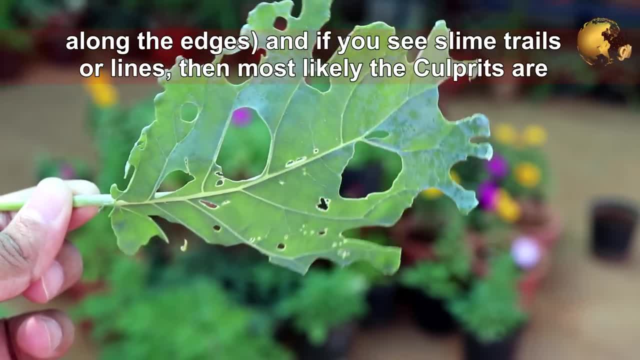 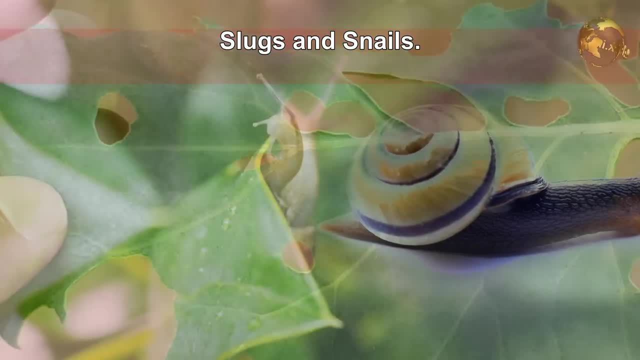 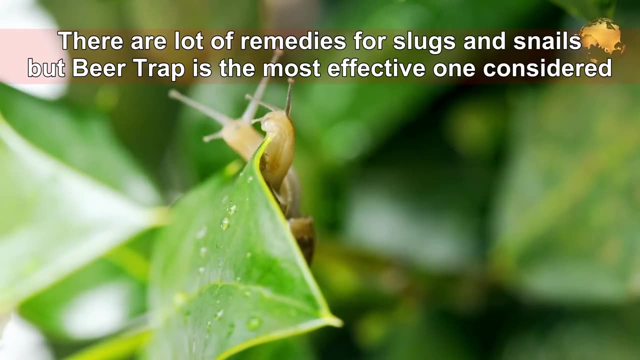 If you see irregular shaped holes in the leaf but not along the edges, and if you see slime trails or lines, then the most likely culprits are slugs and snails. So what's the remedy? There are a lot of remedies for slugs and snails, but beer trap is the most effective. 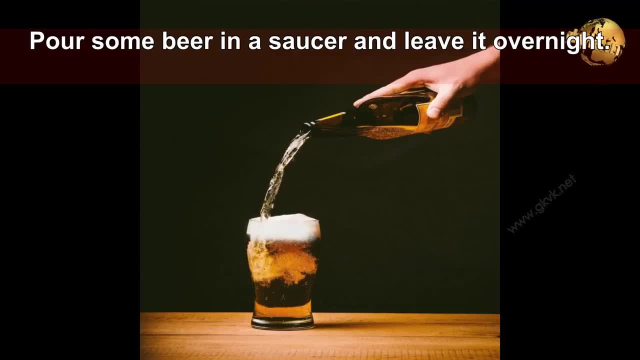 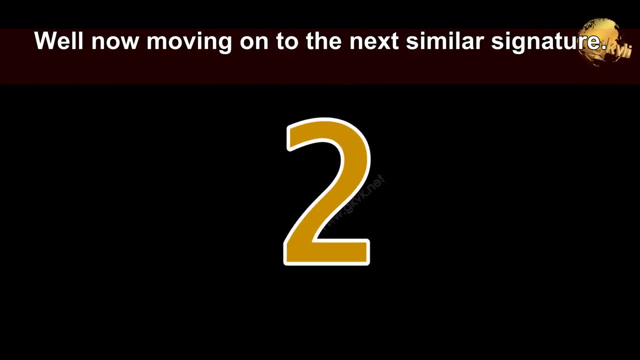 one considered by many. Pour some beer in a saucer and leave it overnight. This attracts and kills these creatures. Well now, moving on to the next similar signature, ie Chewed Leaves Along the Edges. Leaf cutting bees are the culprits. 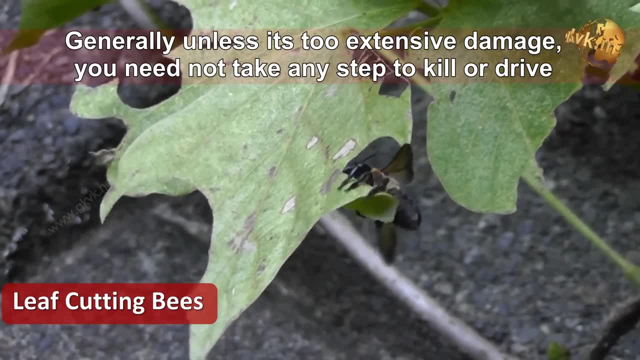 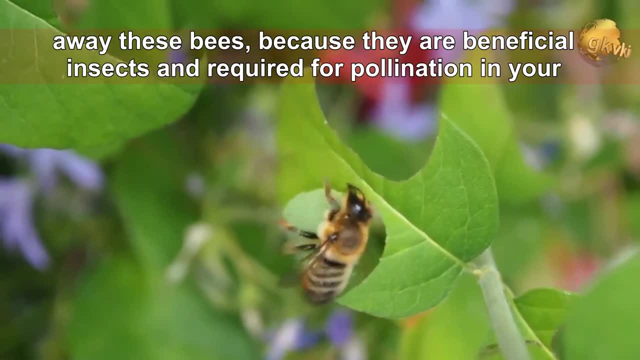 So what's the solution? Generally, unless it's too extensive damage, you need not take any step to kill or drive away these bees, because they are beneficial insects and are required for pollination in your garden. Then the next pattern is Chewed Leaves with Central Leaves. 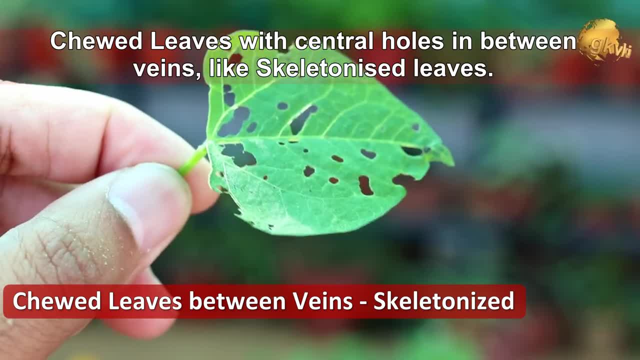 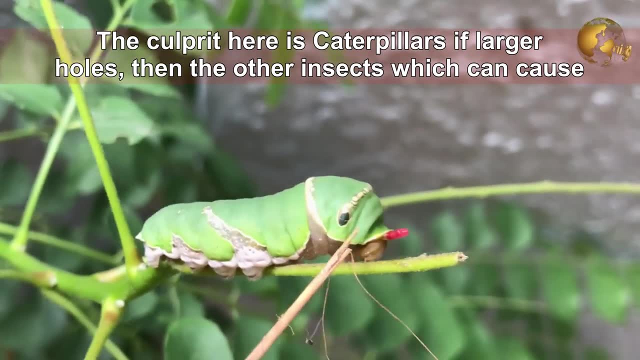 This is a very common pattern. This is a very common pattern. There are central holes in between the veins, like skeletonized leaves. The culprits here are caterpillars, if the holes are larger, and also other insects like beetles, earwigs and sawflies produce this pattern. 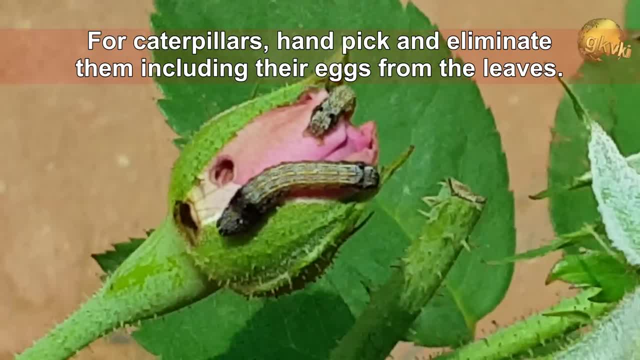 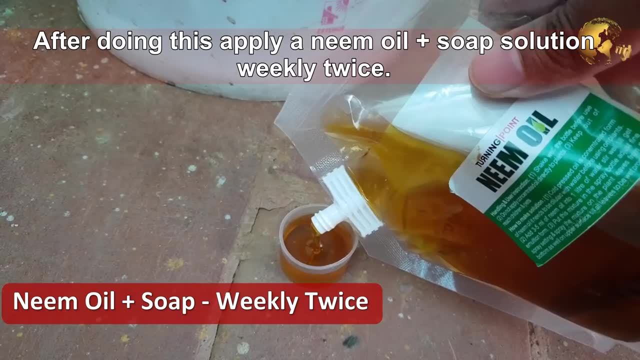 So what's the remedy For caterpillars? handpick and eliminate them, including their eggs, from the leaves. After doing this, apply neem oil plus soap solution weekly twice, ie 10 ml neem oil plus 10 drops of leaf. 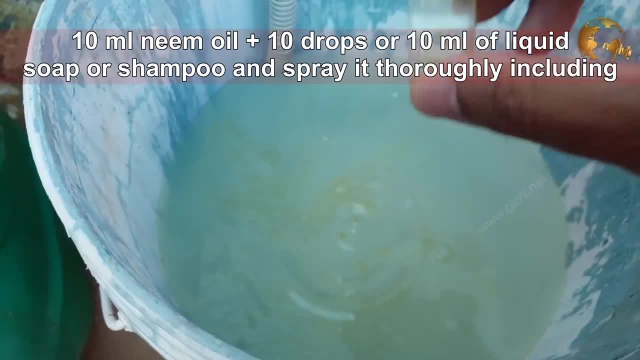 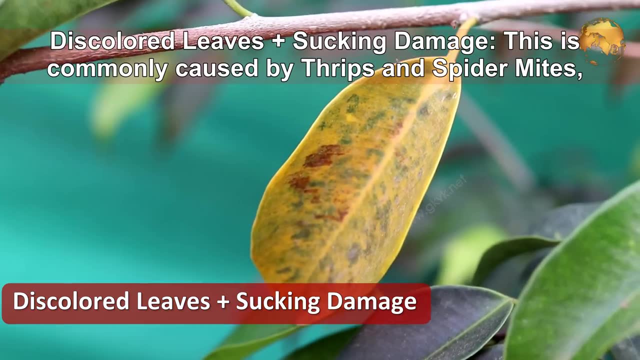 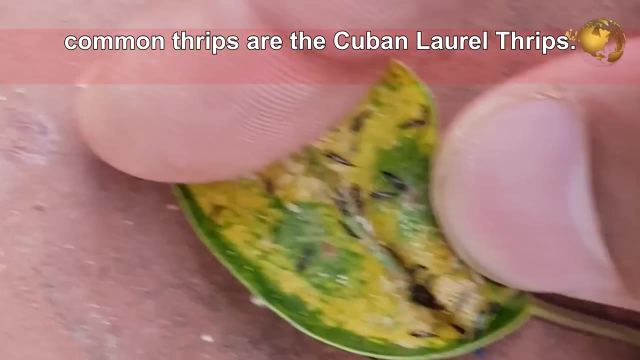 Apply 10 ml of liquid soap or shampoo and spray thoroughly, including the underside of the leaves. Well, the next pattern is Discolored Leaves plus Sucking Damage. This is commonly caused by thrips and spider mites. Common thrips are the Cuban Laurel Thrips. 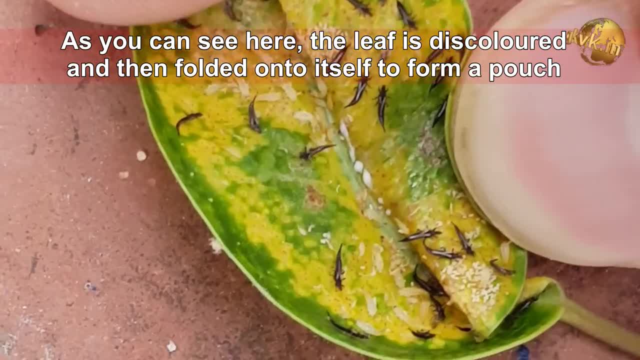 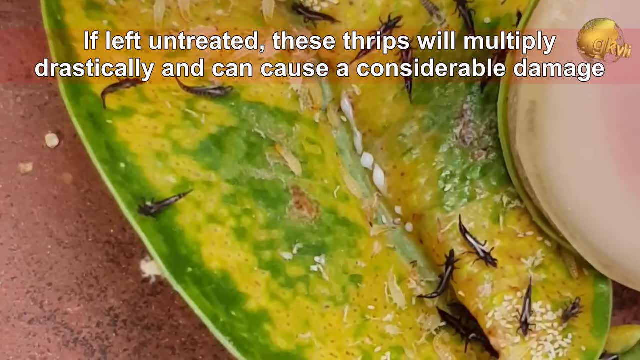 As you can see here, the leaf is discolored and then folded on to itself to form a pouch or cover these creatures and its eggs. If left untreated, the leaves will rot. If left untreated, the leaves will rot. If left untreated, these thrips will multiply drastically and can cause considerable damage. 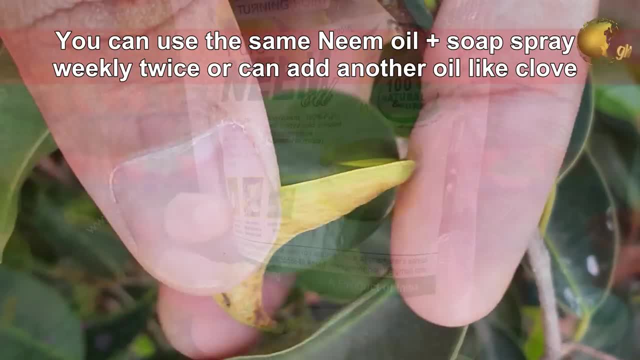 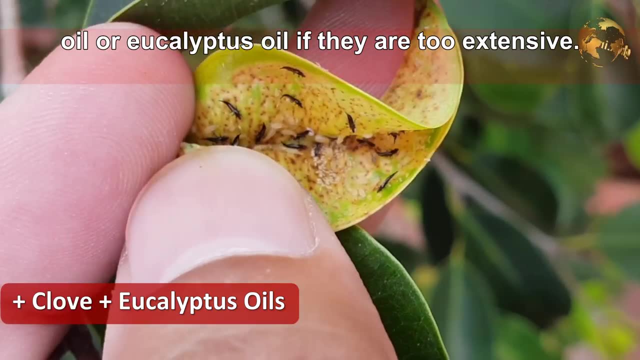 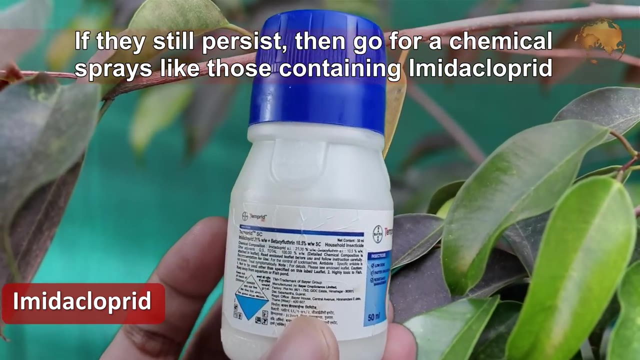 to your plant. So what's the solution? You can use the same neem oil plus soap spray weekly twice, or you can add another oil, like clove oil or eucalyptus oil, if they are too extensive. If they are still persisting, then go for chemical sprays like those containing imidacloprid. 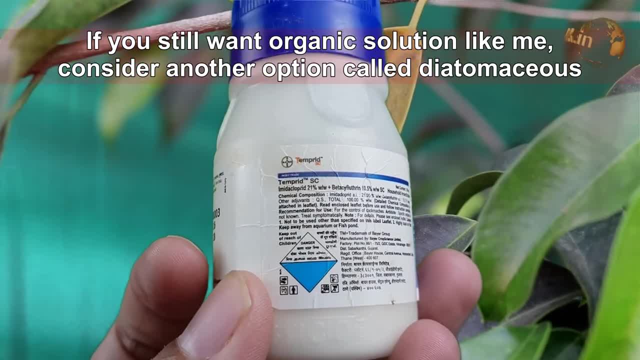 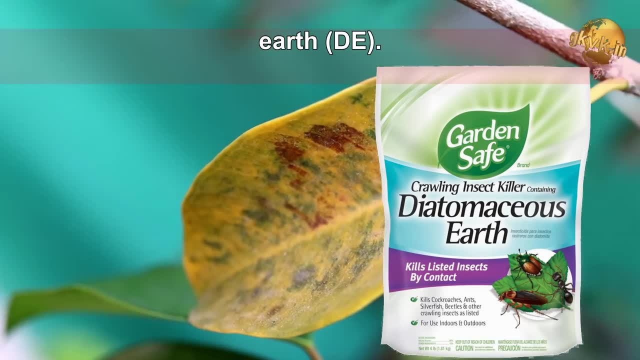 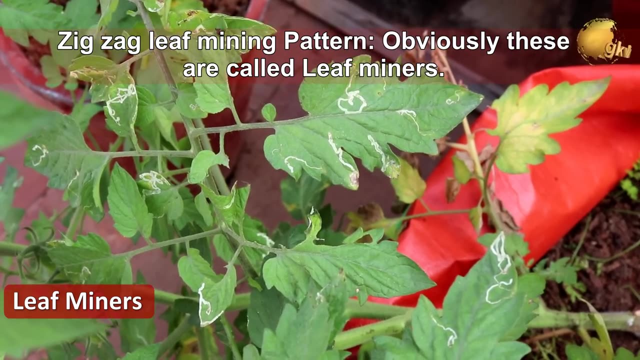 as the last resort. If you still want organic solution, like me, Then you can consider another option called Diatomaceous earth. You can google that or check it at your local store. Then the next pattern is Zig-Zag Leaf Mining Pattern. Obviously they are called leaf miners. 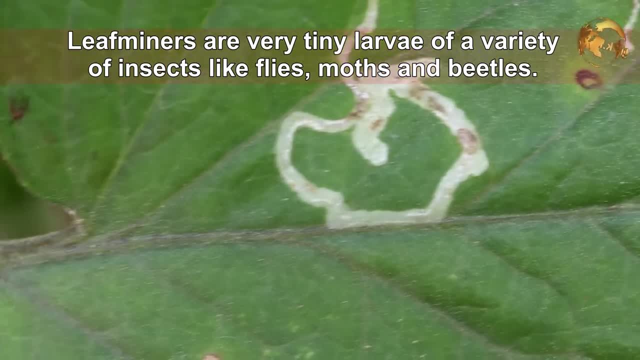 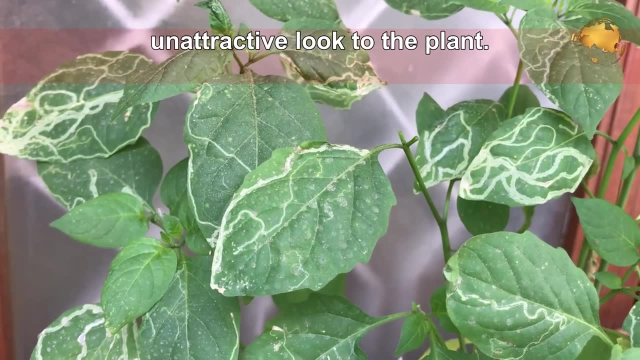 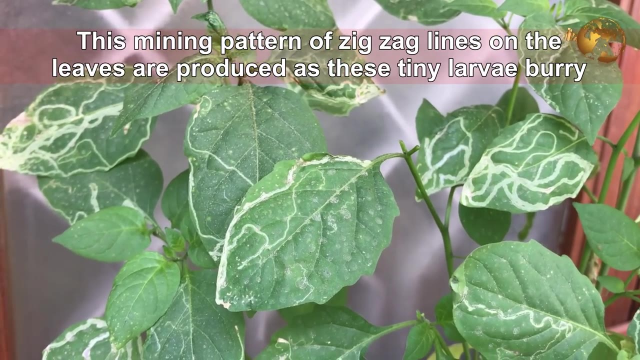 Leaf miners are very tiny larvae of variety of insects like flies, moths and beetles. Leaf miners do not actually cause major injury to the infested plant, but give an unattractive look to the plant. This mining pattern of zig-zag lines on the leaves are produced as these tiny larvae bury. 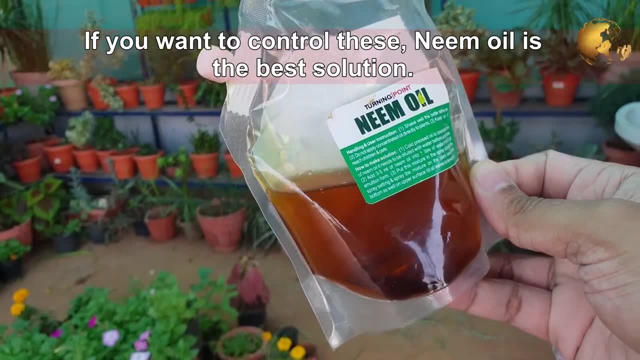 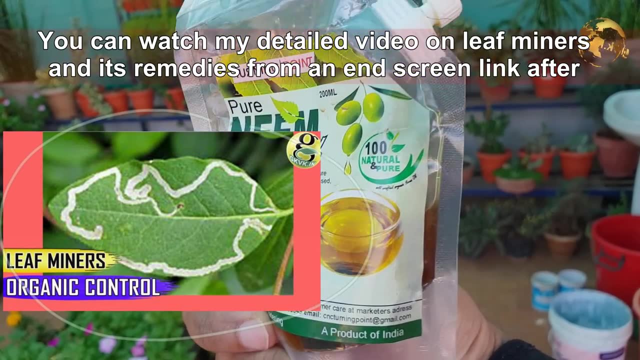 and eat along the infested leaves. If you want to control these, neem oil is the best solution for this. You can watch my detailed video on leaf miners and its remedies from an end screen link after this video. You can also find links to all my related videos on pest control from the description. 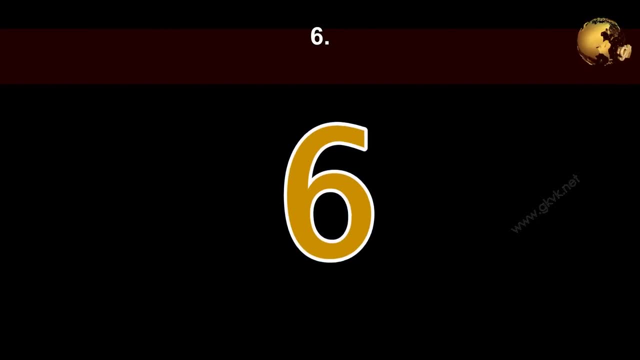 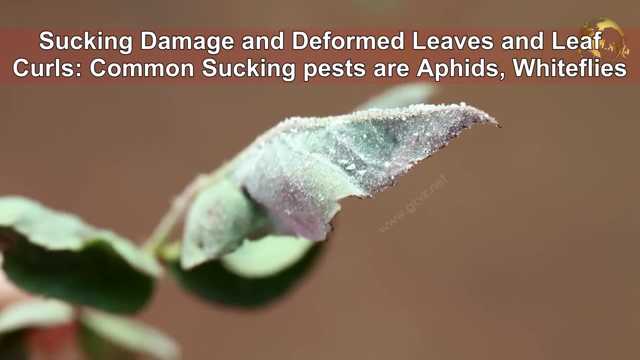 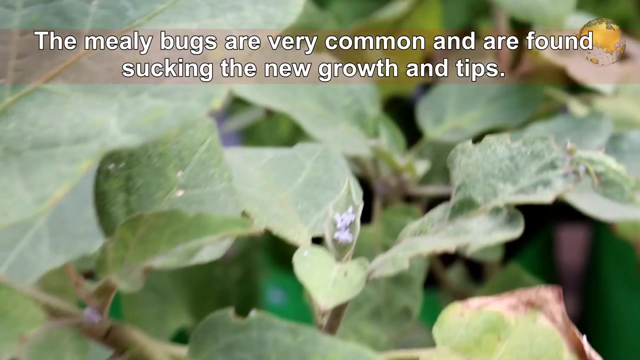 below. We will now move on to the next culprit, ie Sucking Damage and Deformed Leaves and Leaf Curls. 1. Common sucking pests are aphids, whiteflies and mealybugs. The mealybugs are very common and are found sucking the new growth and tips of the plants.